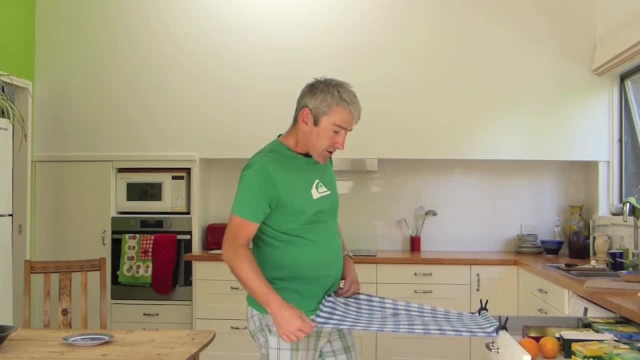 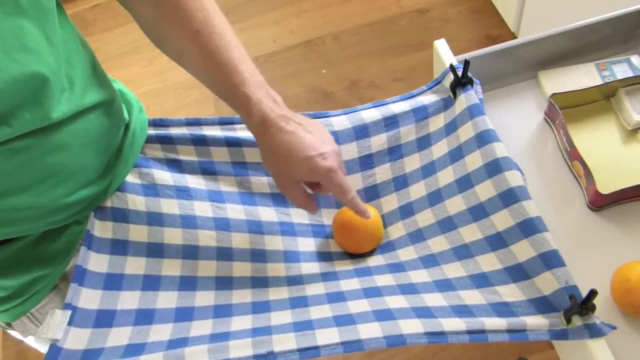 So it might seem to you and me in everyday life that square things remain square. but if you put a heavy enough mass near them, if there was a black hole right here in this kitchen, then suddenly everything would get a bit warped. A black hole warps space in three dimensions. 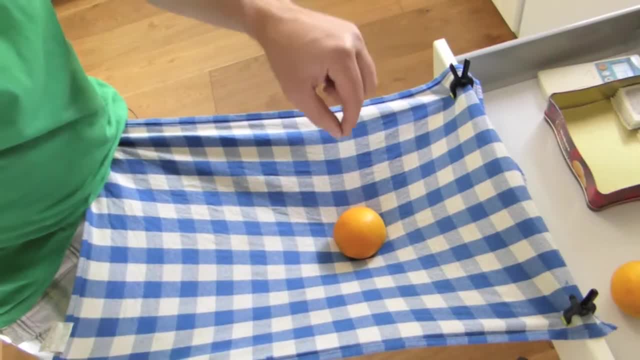 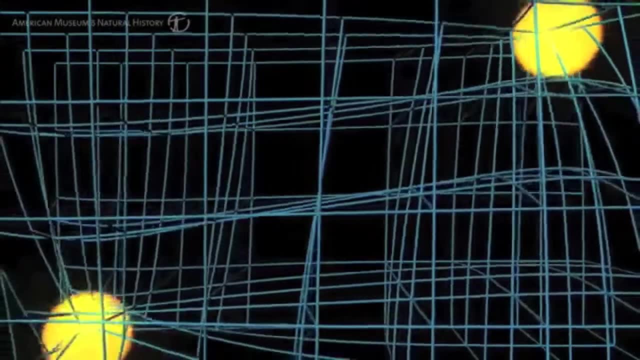 as well. It's kind of hard to get your head around, but you know, of course things tend to roll into it from this direction, that direction, also from that direction and from you know underneath. This is the hardest thing to explain about space-time- Really weird. This has been proven since 1919, five years after Einstein put out his theory. The space is warped around the sun. In an eclipse, we saw a light from a star behind the sun coming around the sun to us at the earth. So the sun is literally. 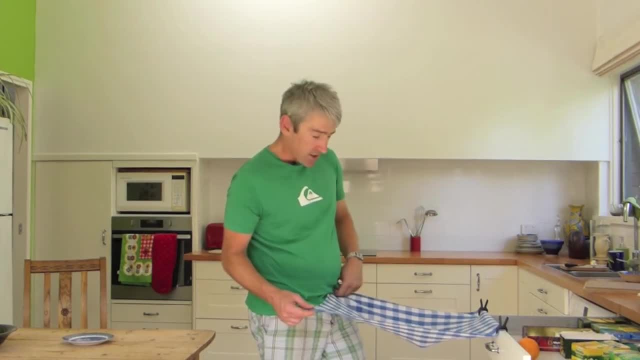 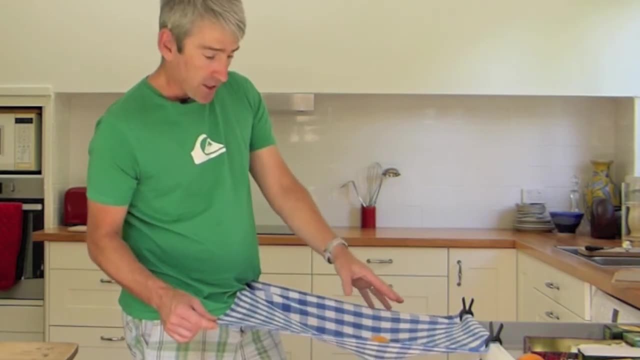 bending space, and it does it to time as well. That's why scientists talk about space-time. So when things sit there by themselves, they don't really make gravitational waves. they warp space, So not until something violent happens. like you know, they move around, or? 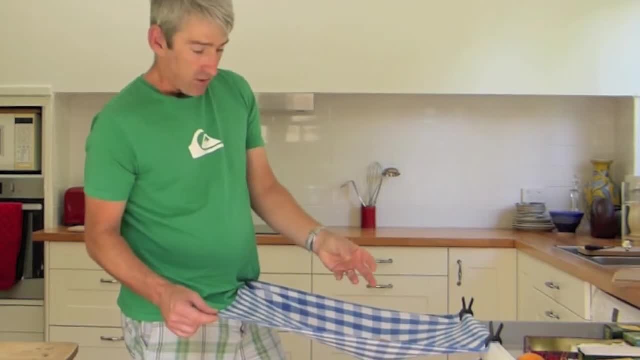 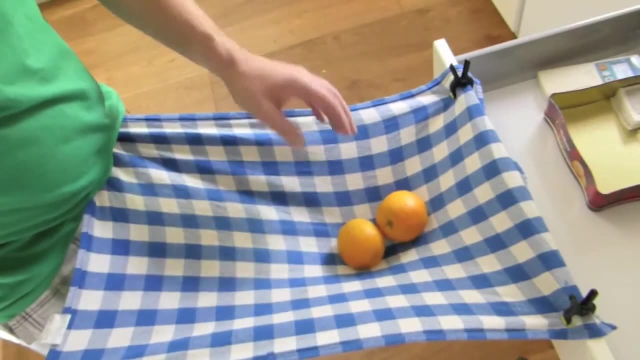 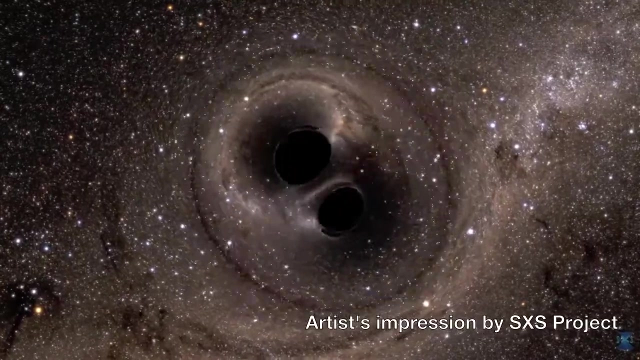 suddenly land. but masses don't like suns don't just appear out of nowhere. Everything happens quite slowly, unless you get a collision, And that's what the scientists observed: A couple of black holes colliding And that, as you can see, makes all of space quiver. 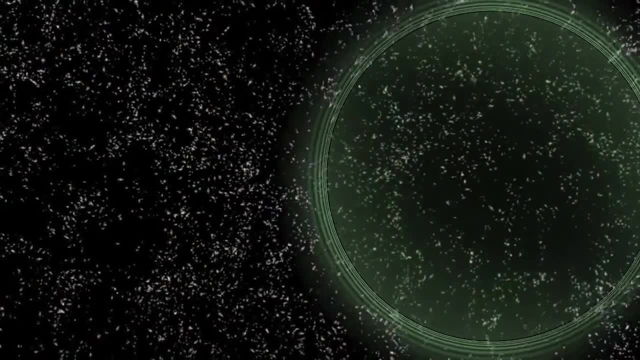 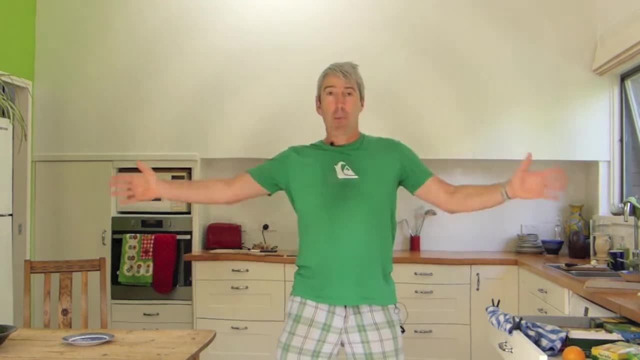 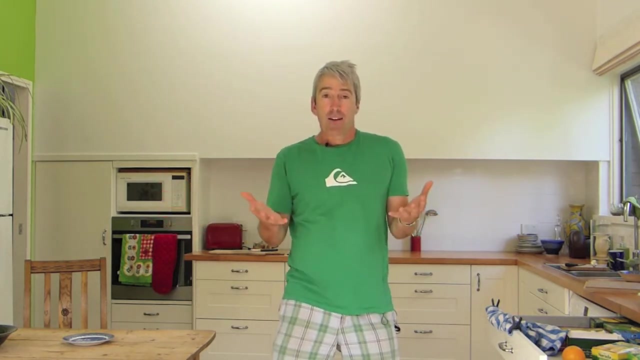 Waves in space travel right to us, where we can see them. So right here a gravitational wave can come through and actually warp space. See for a moment, there I got taller and thinner and then I got shorter and fatter and then I went back to normal And that. 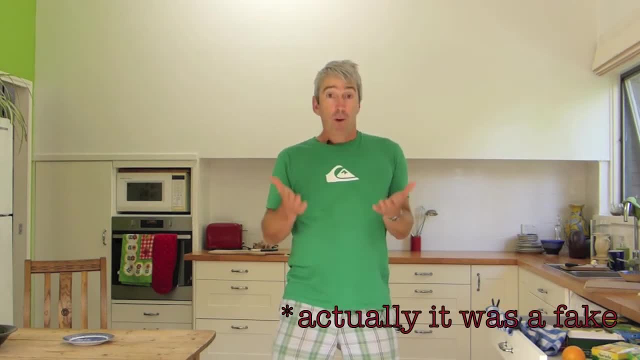 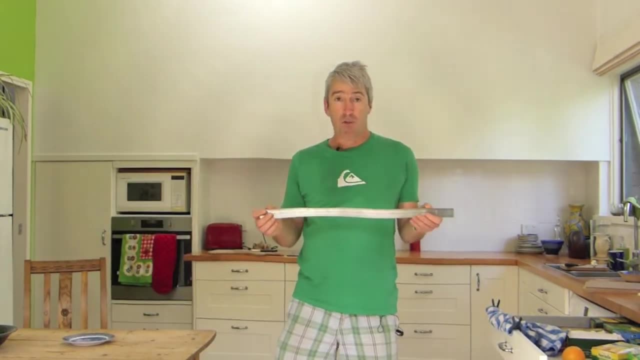 was a gravitational wave passing through. But the really hard thing is: how are you going to measure it? Because if you have a ruler, as a gravitational wave passes through, it stretches as well, So you can't actually see it measuring. The only thing that you can use is light. 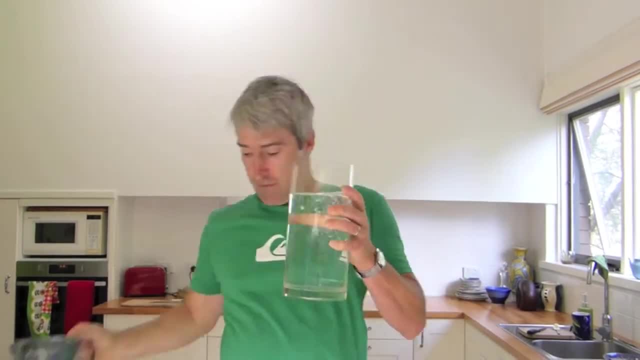 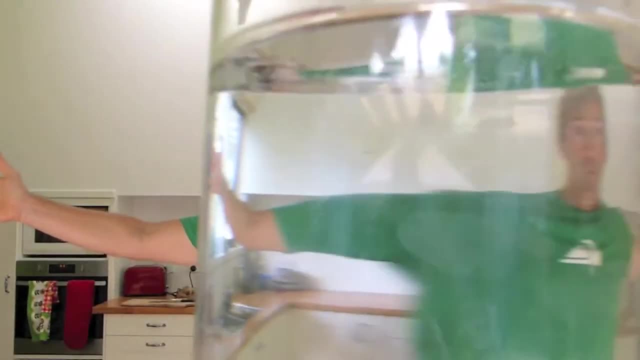 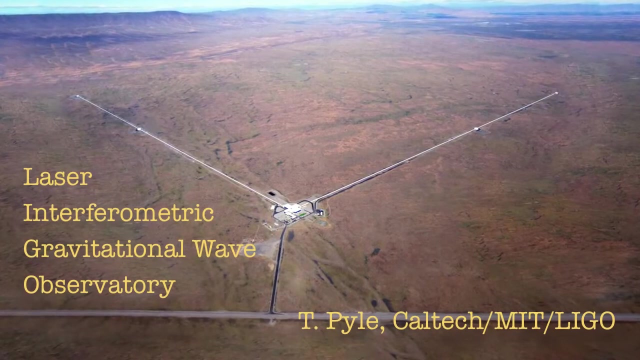 It's a little bit light. A black hole would warp space, kind of like that. The only thing you can measure it with is light, And that's where LIGO comes in. They've used laser beams between two mirrors, bouncing backwards and forwards. Got another set.